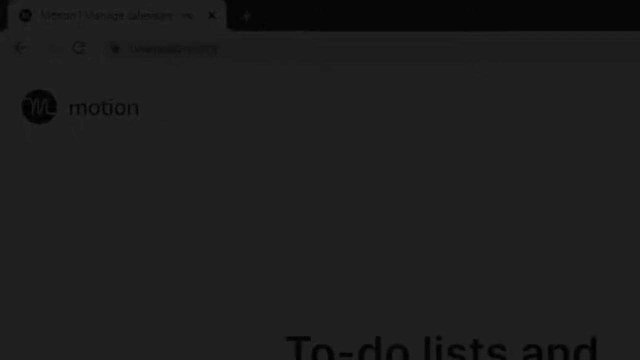 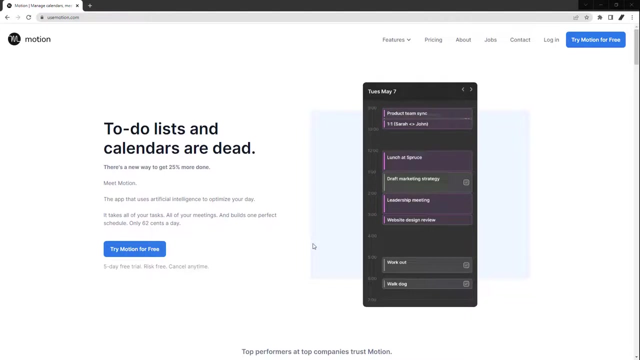 long time, But no app has features like Motion. This is Kalali and we'll be doing Motion Review. Motion is an AI calendar app. With this app, you can manage your entire life. It can track your schedule, recurring tasks and meetings. 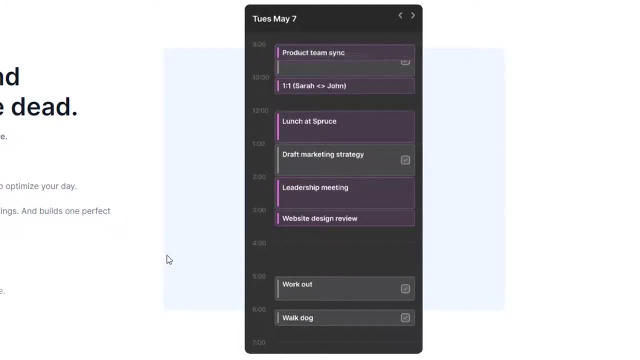 The AI feature automatically plans your day based on variables such as deadlines, working hours, task length and resource meetings according to a calendar. Motion lets you know about users and their preferences. It also helps you understand your schedule and manage it better. The Motion app is very simple. When you first start, you are prompted to connect your calendar. 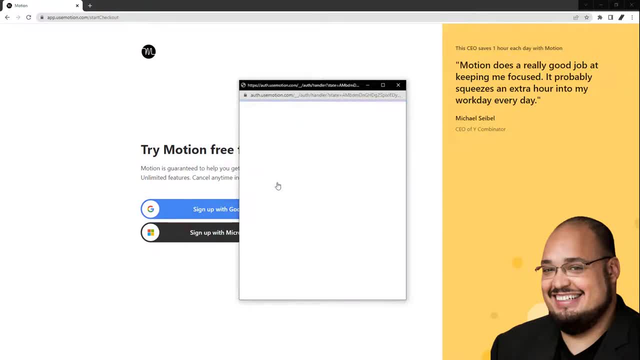 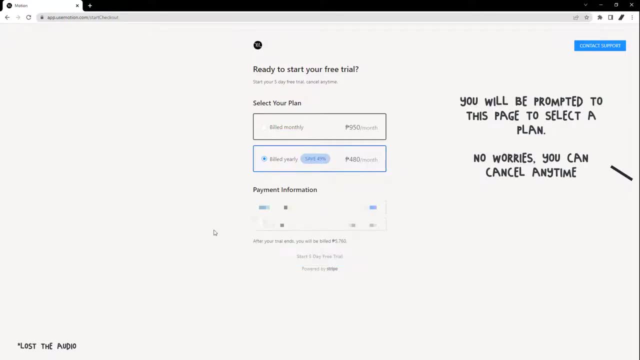 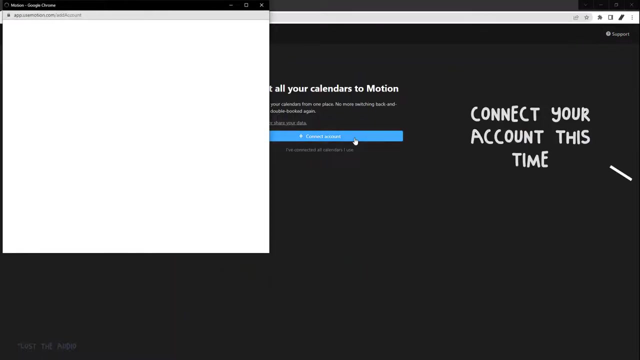 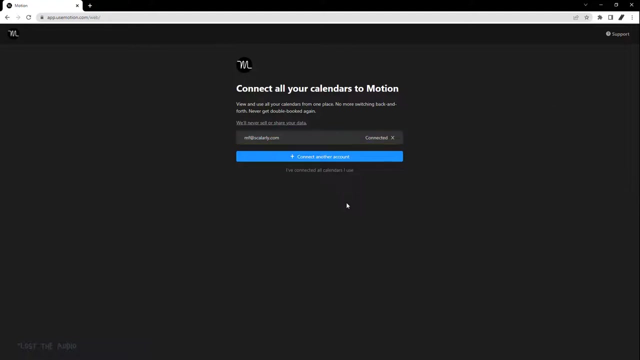 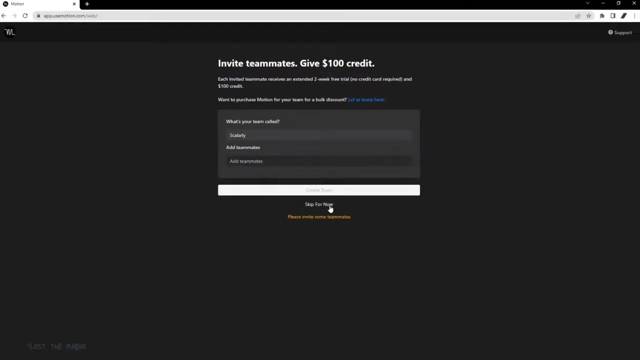 of choice. It's either Google or Microsoft, because those two are the only ones available at the moment. You can also use the app to manage your schedule. You can also use the app to manage your schedule In the event you don't actually want to a首. Tusk is Katalk YouTube. Use the app on time, as Sara has beenly has beenmelding the calendar configuration for her 3 days, But it can be a bit more challenging using the app. The good facts about this app is that it can do 2 workday plans across 3 days. So when you are trying to plan out a schedule- In the case I have set up a 7 day 2019 schedule- if I decide to bring in 3.5 people at a certain length, If that's not that easy, I'd recommend you go to The bees, but I do not do the 15 day. schedule so it won't take much trigger to drag them in to it. On the other hand, we can preferably arrange couple days to even have the schedule set specific out for your current schedule and over time. First, it allows you to find the schedule and organize the schedule. 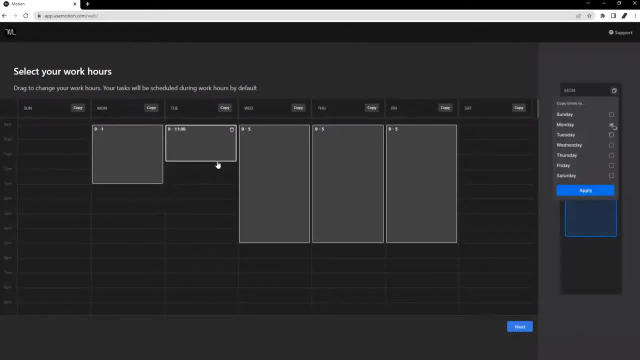 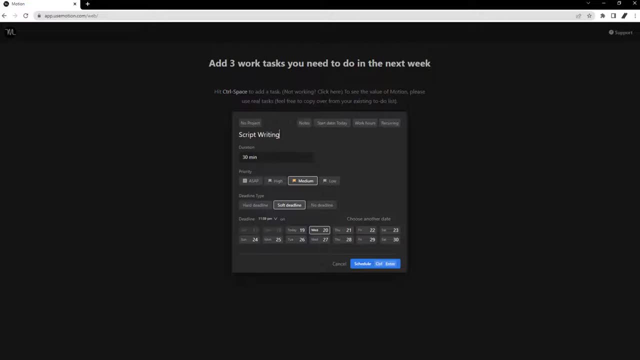 You will also set your work hours in this step, which is the timeframe that Motion will add work-related tasks. You will also add your recurring time blocks and tasks like launch, replying to emails and weekly team meetings. I'd suggest getting comfortable with the UI and going through the settings to perfectly. 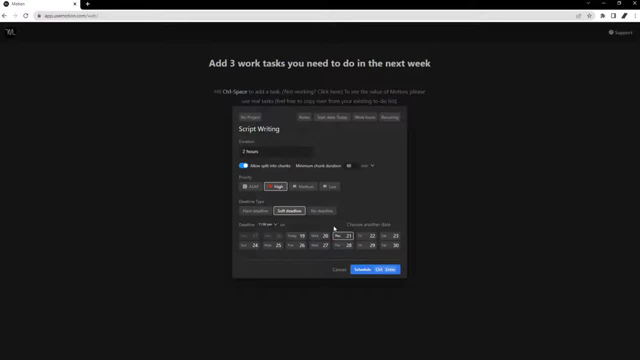 tailor the app for your needs before adding all of your tasks. Motion has three main features, which are tasks, calendars and the booking system. All of the tasks and meetings you book will be added to your calendar and sorted by the app. 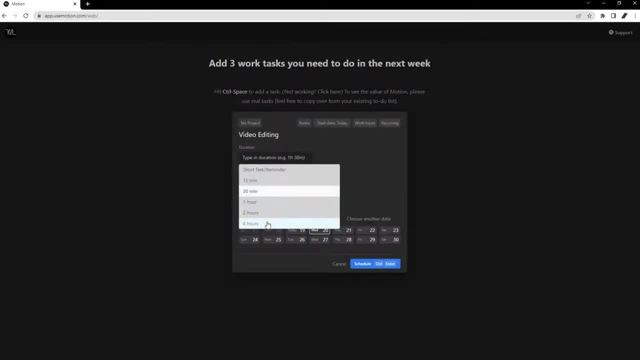 Motion is available as a web app, mobile app and Chrome extension. Really get the most out of Motion. you need the extension to use the shortcuts. After integrating your calendar accounts and getting comfortable with the app, you should start adding your tasks, which Motion will automatically plan in your calendar. 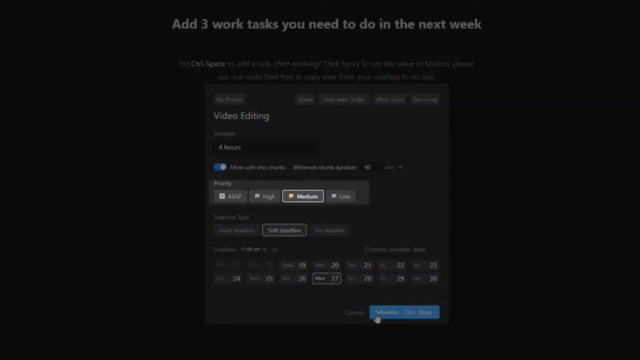 Tasks are planned around many factors, which are priority, ASAP, hard deadline and soft deadline, The deadline date, start date and when you can work on the tasks, like work hours, whole day, nights, mornings and any other schedule you create. 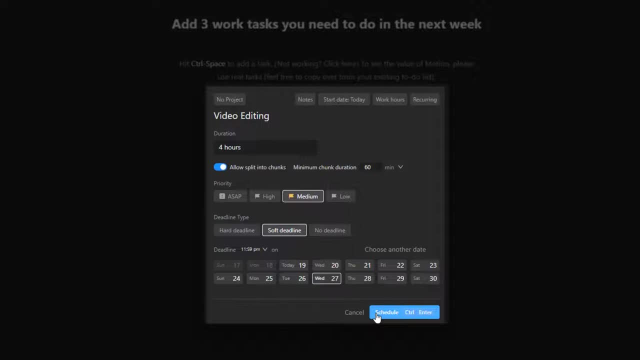 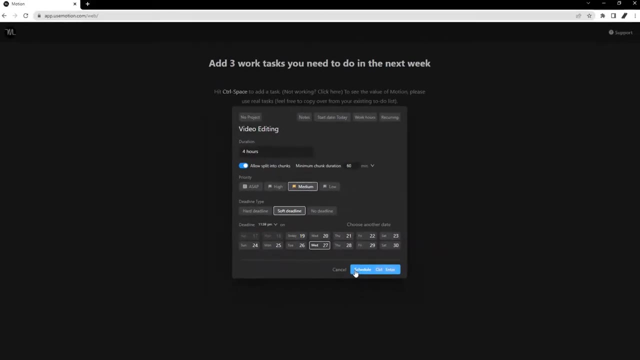 Using the variables mentioned, the app can help you prioritize tasks efficiently and make sure everything is done before their respective deadlines. You can also sort tasks into projects to better understand where your time goes. To create a new task, use the control or command for Mac plus paste shortcut from any webpage. 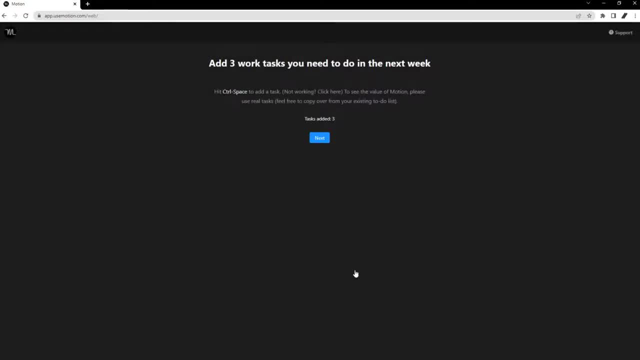 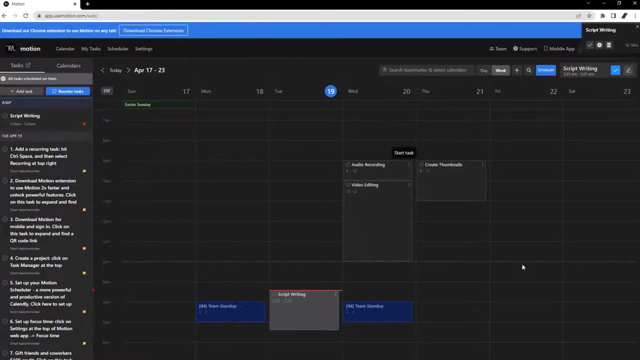 if you have the extension, As you add more and more tasks, you will be able to create your own tasks. As you add more and more tasks to the app, you will start to notice your calendar filling up. However, you may notice your tasks and events are color-coded within the app. 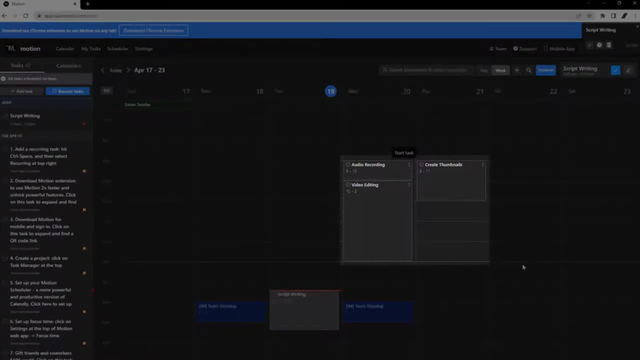 Gray blocks are tasks created within the Motion app and there are two types of tasks which are differentiated by their borders. Dotted borders indicate a free task, which means that there are other timeframes where the task can be completed before reaching the deadline. 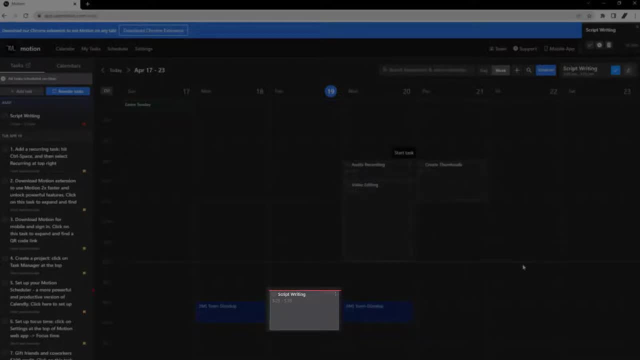 If a task has a full border, that means that it's a locked task that should be completed at the specified time to be ahead of the deadline. Different color tasks are tasks that have been imported from your integrated calendars. If you would like to change the timeframe of a task, simply drag the task block in the 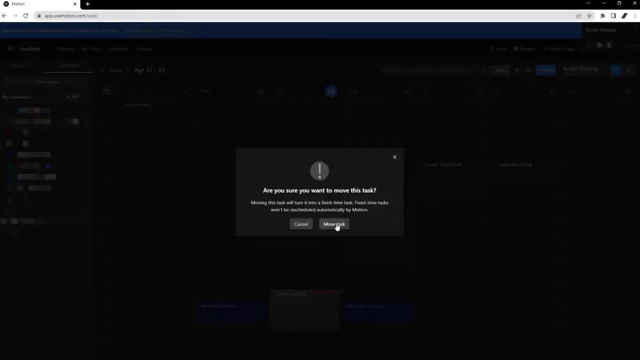 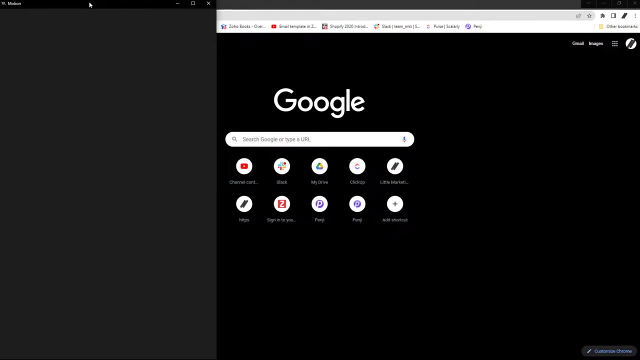 calendar to your desired time. However, this locks the task in time, which means the app won't be able to change its placement on the calendar. You can view your calendar from anywhere using the Chrome extension by pressing Alt plus C on your keyboard. 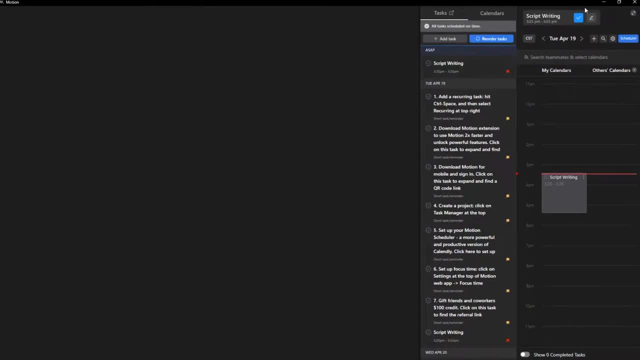 And when it comes to privacy, Motion won't disclose the name of a task on your personal account. You can also change the name of the task on your personal account. You can also change the name of the task on your personal account. You can also change the name of the task on your personal calendar to other team members. 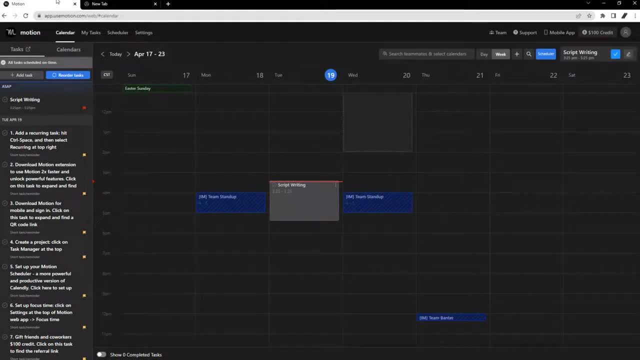 unless you change it in the settings. If your industry requires you to book a lot of meetings, then this feature should be useful. You can create booking pages like Calendly, but with fewer features, and the time booked will automatically be added to your Motion calendar. 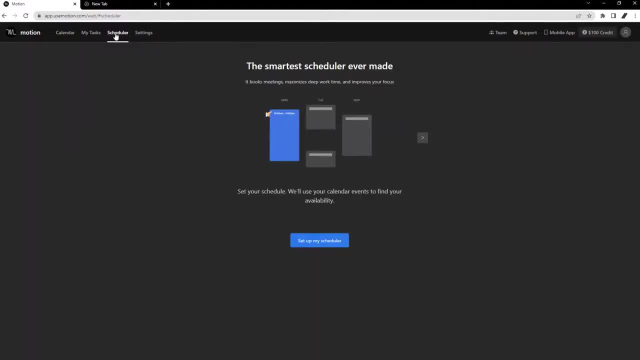 Within the Scheduler tab in Motion, you can create: click and drag on your calendar to create time blocks that you want to keep free for meetings. Finding a shared free time where you can have a meeting can be a great way to create time blocks for your meetings. 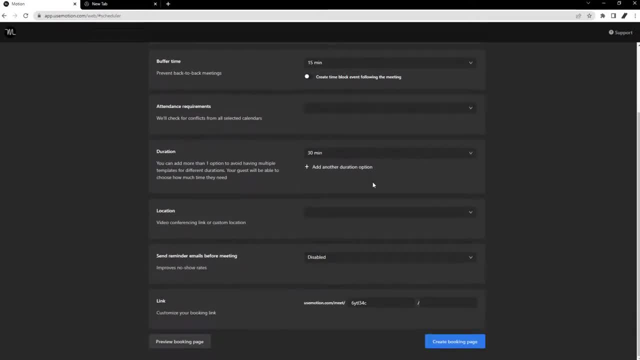 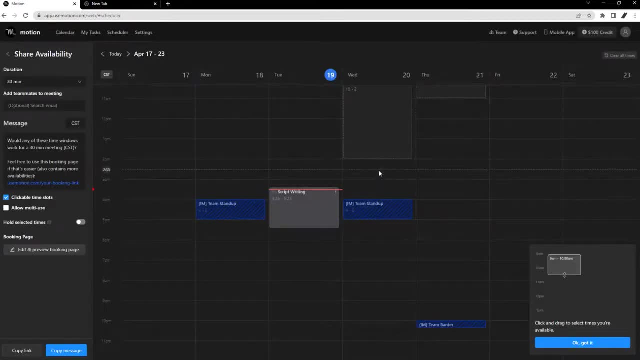 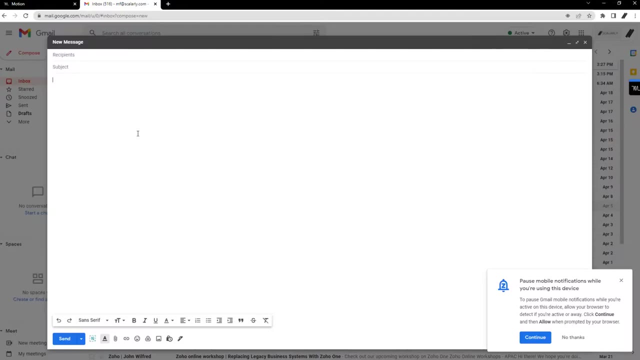 Using the Template Maker in Motion can be a lifesaver if you're ever in this situation. The Meeting Assistant works as follows: You pick times when you are available and ready to host a meeting And, using the Alt or Option plus A command, you can create a message pre-filled with the 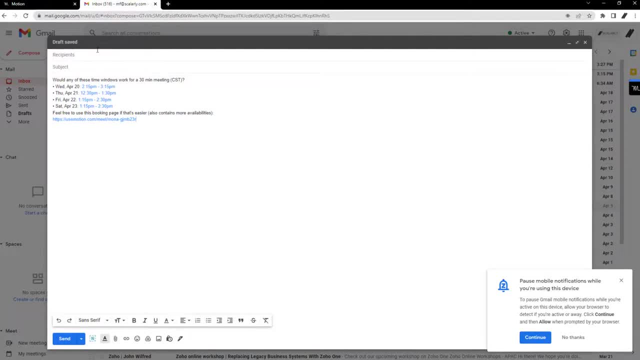 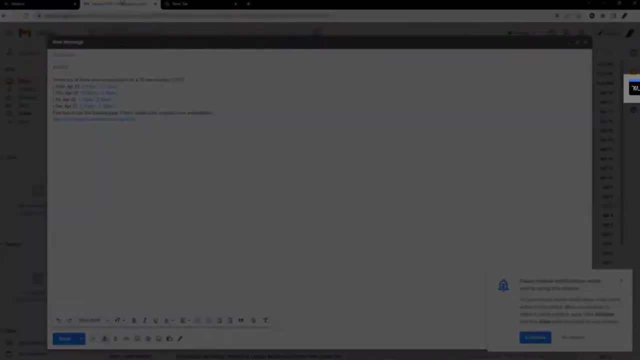 available time frame that you can send to a client and the booking page link. The Chrome extension adds a small widget to the side of your web browser where you can view your calendar tabs, etc. You can add tasks, share available times, go to the web app and contact support. 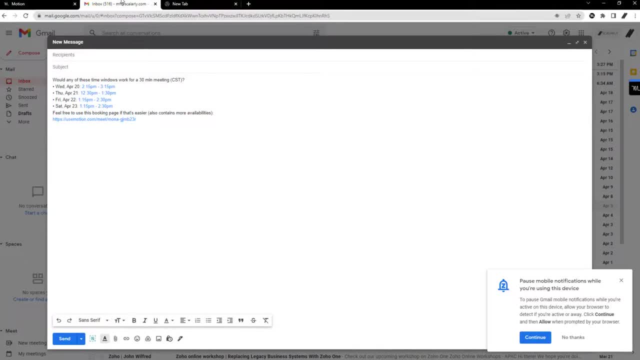 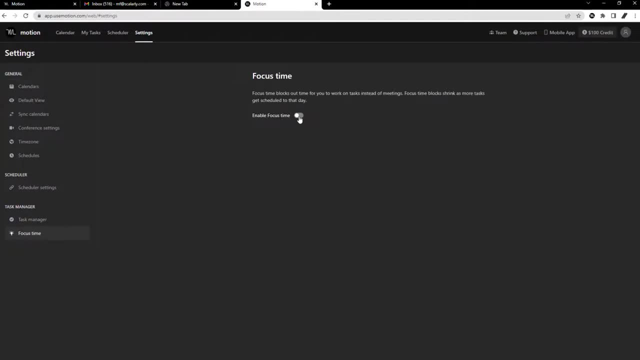 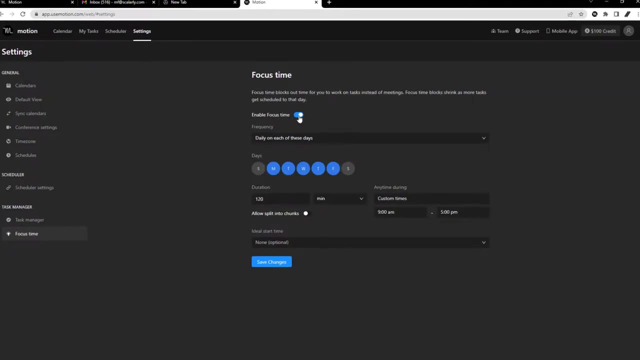 The Chrome extension also enables keyboard shortcuts that will make your workflow undeniably faster when adding tasks and viewing existing ones. Their anti-destruction system also keeps your time on social media concise and productive. It helps you stay focused with alerts and their sophisticated destruction removal system. 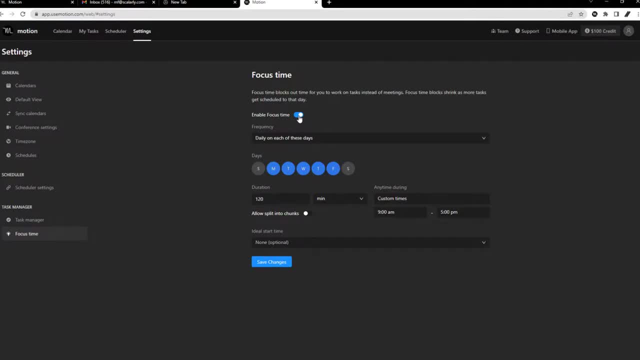 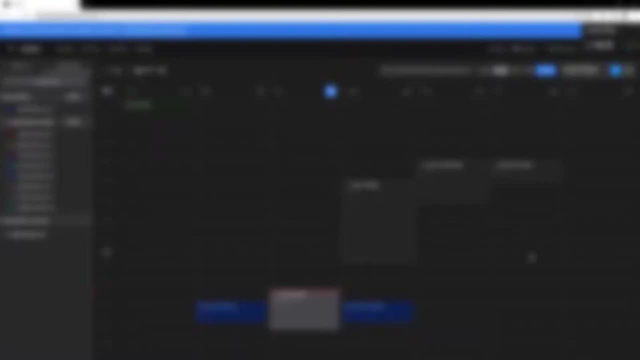 is superb. At first glance I really liked the tool, But the more I used it, the more I noticed the difference. I think it's a great tool. It's easy to use. It doesn't require enough practice. The feature features are missing that are a staple of most productivity apps in this. 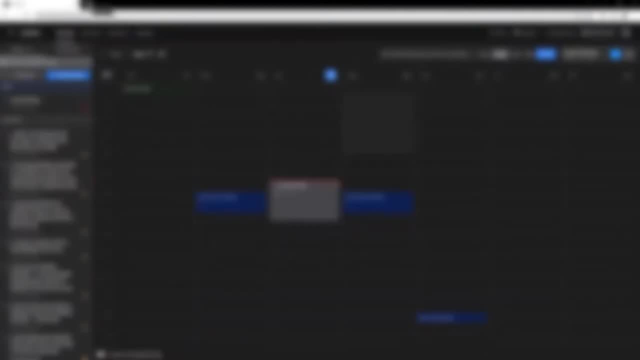 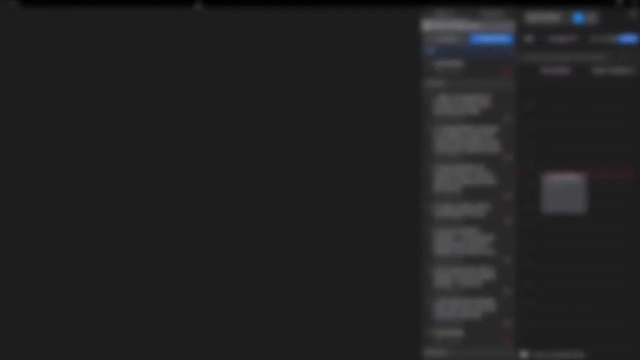 age. Small things like color coding tasks created from the app are not available. Importing tasks from other apps like ClickUp would be nice, without having to go through Google Calendar would also be appreciated. The Motion app is still in development And you can certainly see that when navigating the tool. 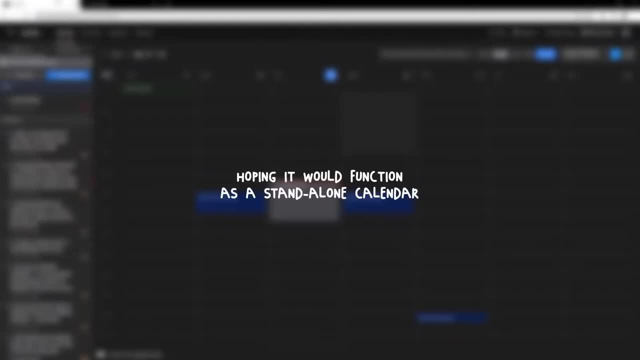 But I wish it would have been able to function as a standalone calendar, not just an extension to Google or Outlook. The price for Motion is $34 per month, which is enough when you make two apps at once right month, which is steep, but you can pay $19 per month if billed annually.